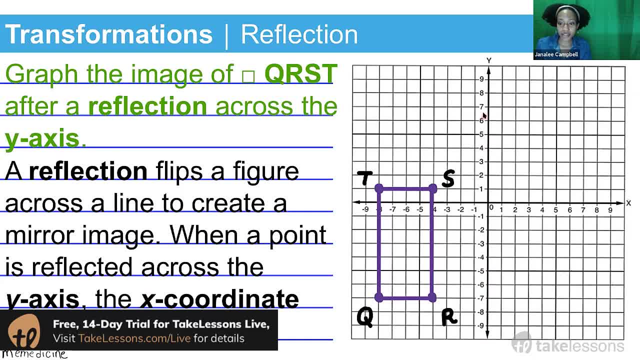 All you're going to do, basically, is change the sign of its x-quartetto. When a point is reflected across the y-axis, all you're going to do, basically, is change. so we're flipping about this line here, the y-axis line of the two-dimensional. 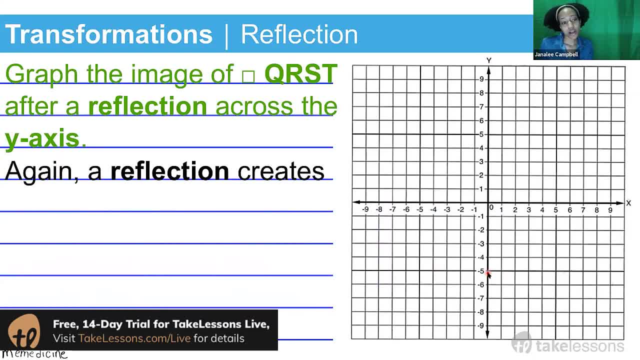 coordinate plane. okay. so again, just for reiteration, a reflection creates a mirror image: Q, point Q is eight units to the left of the y-axis. okay, and remember the negative in front of a position or an X. a position on the x-coordinate just means you're to the left of the origin. so I don't want people to get. 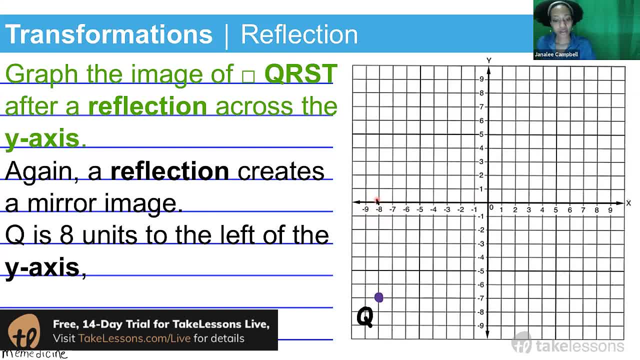 intimidated when they see negative signs. alright, so again we see our points. Q is eight units to the left of the y-axis. its reflection is obviously going to be eight units to the right of the Y axis, so let's draw that right now. All right, so a reflection is basically equidistant. 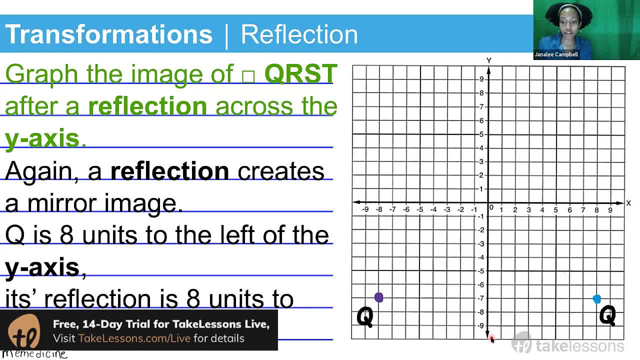 about whatever axis, you are doing your flip over And we're doing our flip over again the Y axis, And it's not Q because we have shifted its position. so we're going to call this Q prime to denote that it's been transformed. 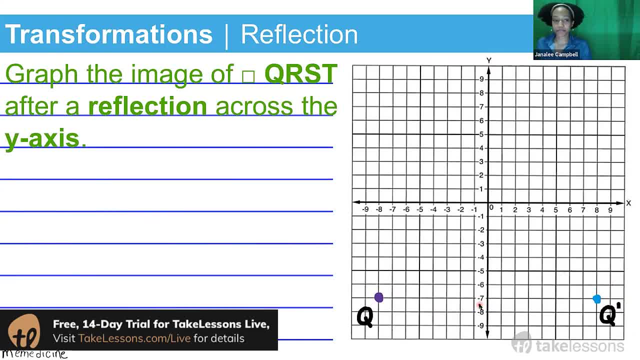 via reflection about the Y axis. Now in our original figure we had point R. Point R is located four units to the left and seven units down, so it's at position negative four and negative seven, and again we're going to reflect it across the Y axis. 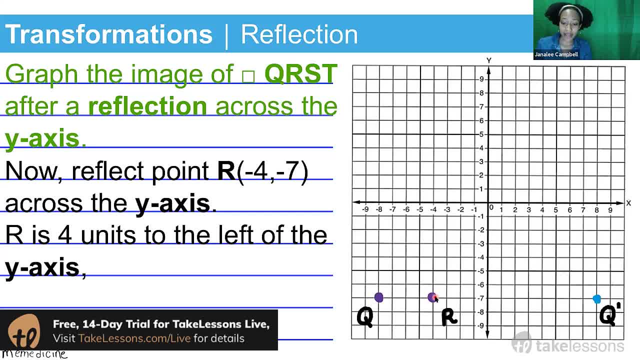 So, since R is four units to the left of the Y axis, to flip it about the Y axis, all we have to do is shift it four units to the right because, again, when you're flipping or reflecting about the Y axis, all you're doing is moving equidistantly. 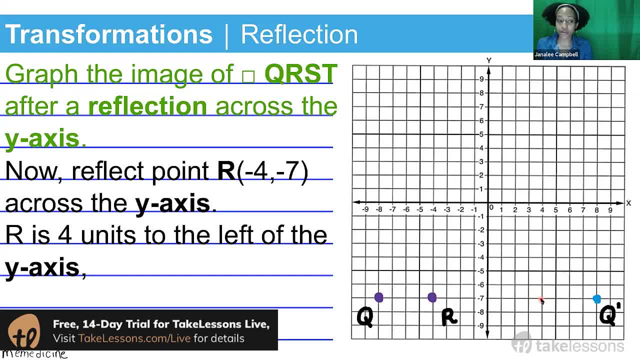 with respect to the Y axis, and in order to do that, all you're going to do is change the X coordinate. Okay, so its reflection has to be four units to the right of the Y axis, And this is going to be R prime. 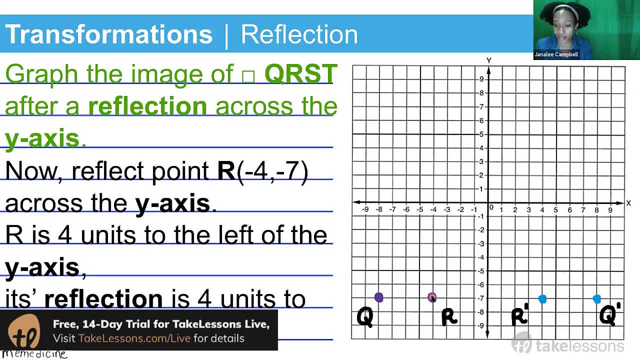 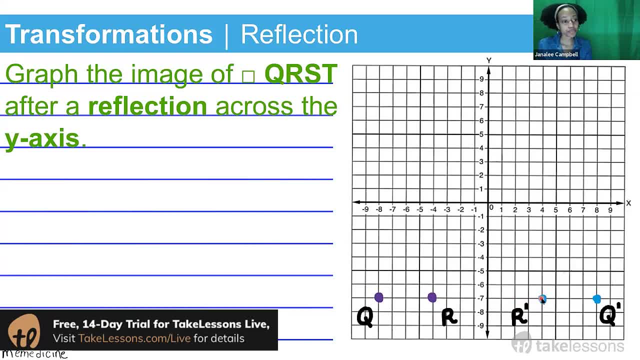 because we shifted our original figure, or point R, through reflection on the other side of the Y axis. Now we're going to reflect point S. okay, So we're on our third point of our original rectangle. we're going to reflect it about the Y axis. 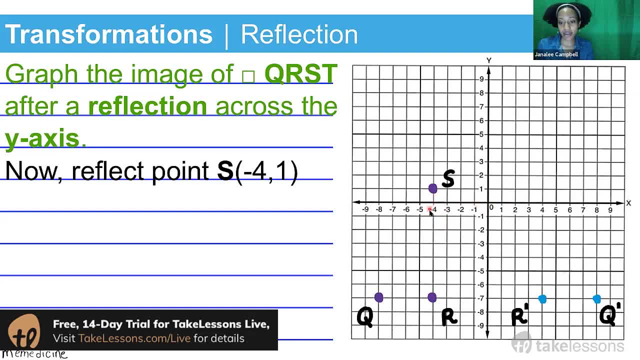 It's located horizontally at negative four, which means we had to travel four units to the left of the origin. Recall: the origin is located at zero, zero And it's shifted upward one unit, so it's located at X equals negative four, Y equals one. 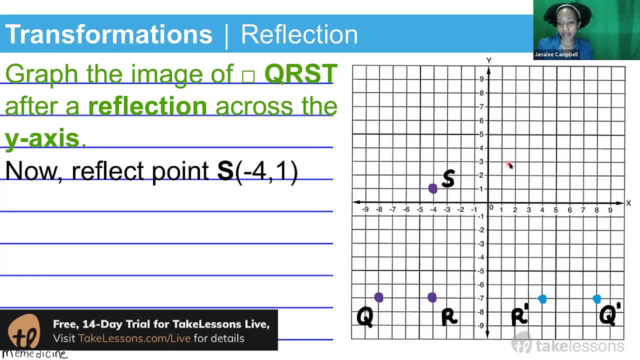 Okay, And to flip it about the Y axis, we're just going to shift it equidistantly with respect to the Y axis, And I'm supposed to be at four. yeah, So we're over here at four, And so if S is four units to the left of the Y axis, 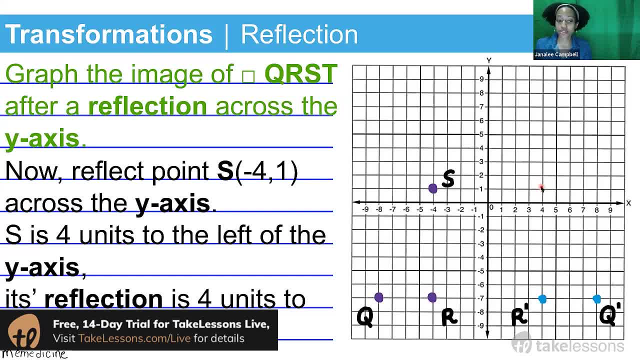 to reflect it. we have to move it four units to the right of the Y axis, And I'm just going slow. I know this might be redundant for many of you. I'm just going slow Because there are some people in here who are not really familiar. 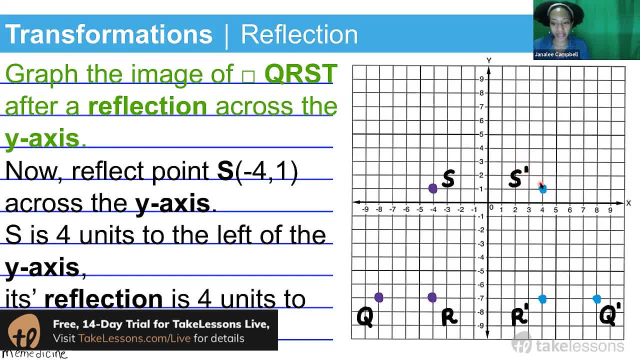 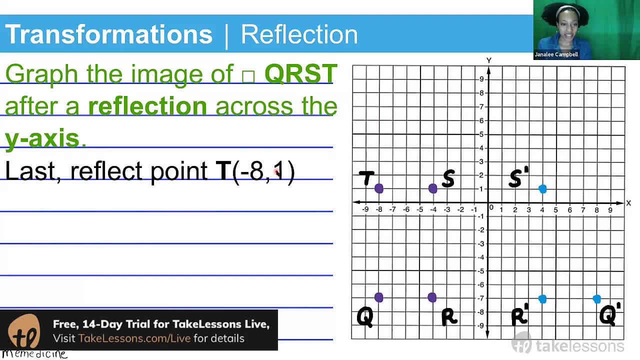 with navigating the coordinate plane. okay, All right, but last but not least, we're finally at point T. Okay, so point T is located eight units to the left of the origin and one unit up, And so we're going to reflect it across the Y axis.